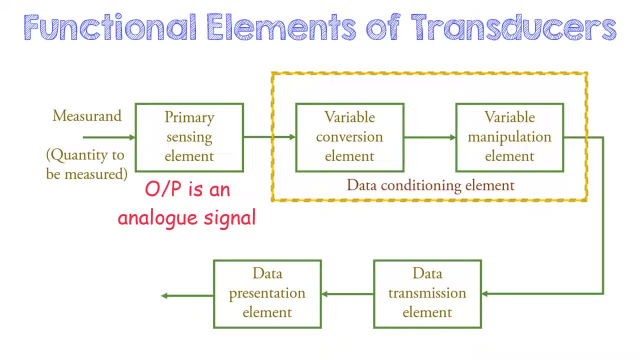 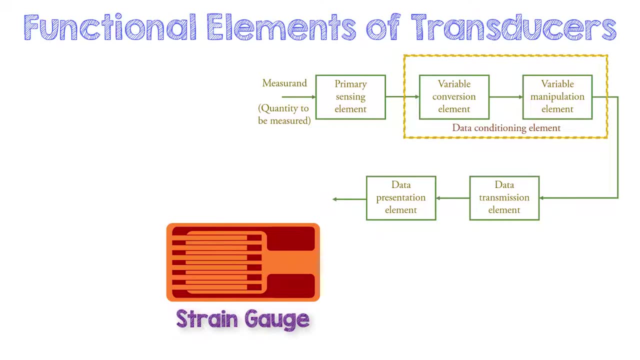 element converts the physical quantity under measurement into an analog signal. The example of such an element is a strain gauge. Strain gauge is a device used to measure load or force. As the force is applied to the strain gauge, it gives change in resistance. The 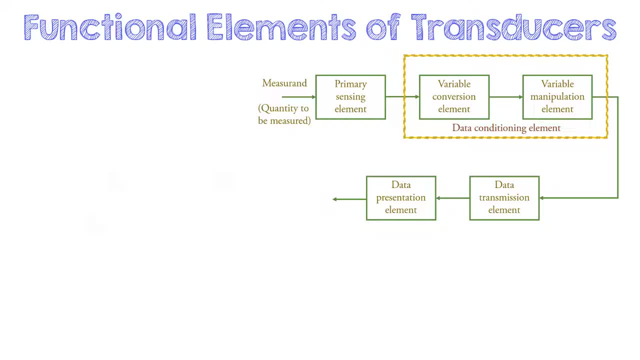 next block is variable conversion element. This block converts the output of primary sensing element into a suitable form without changing the information about the physical quantity under measurement. Taking the previous example of strain gauge, we know that strain gauge gives the data of force applied as a 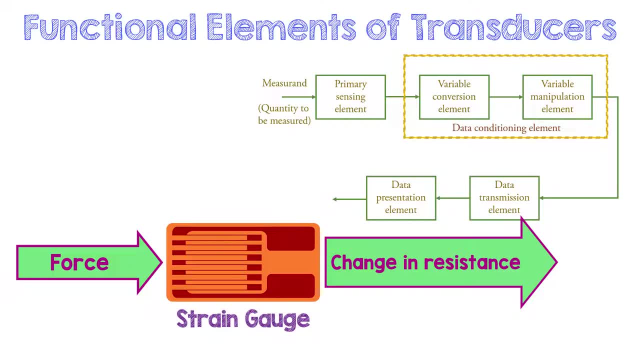 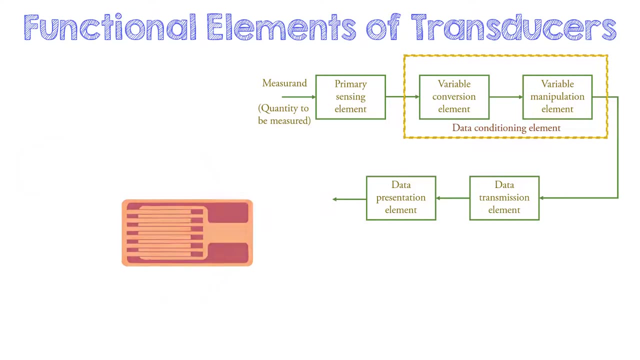 change in resistance. However, this change in resistance cannot be used directly to know the value of the force applied. The change in resistance needs to be converted into an electrical quantity to be easily measured. For this, a Wheatstone bridge is employed By connecting the strain gauge to one of the 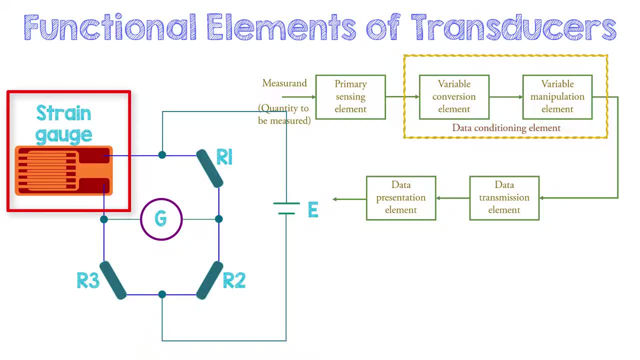 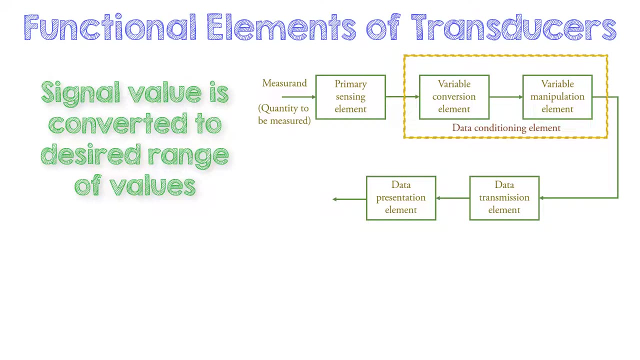 arms of Wheatstone bridge one can convert the change in resistance to voltage. The Wheatstone bridge is an example of variable conversion element. The next block is a variable manipulation element. Here the signal values is changed to get a desired range of value, Generally the accepted signal. 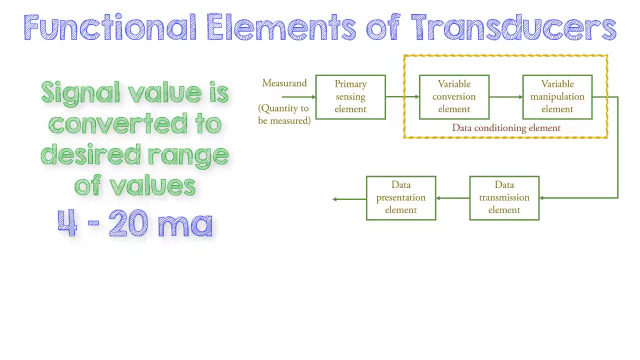 ranges in any process industries are 4-20 mA, 0-5V or 3-15 psi. Variable manipulation element can help one achieve these standard ranges using signal conditioning circuits. The next element is the data transmission element. This block is responsible to transfer. 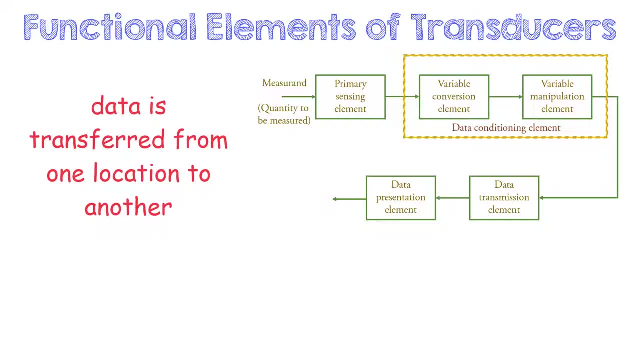 the data from one location to the other desired location. The transmission parts that can be used are pipes, electrical cables or radio links. The last element is the data presentation element. This block is responsible for recording and displaying the measured values to the operator. Examples of this can be analog meters.